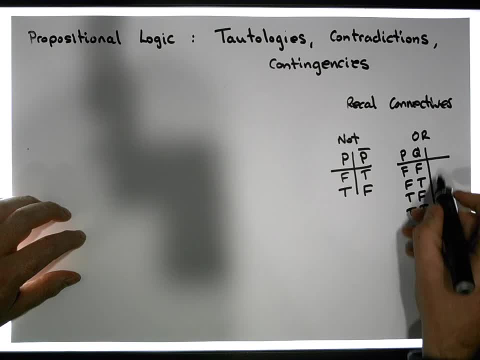 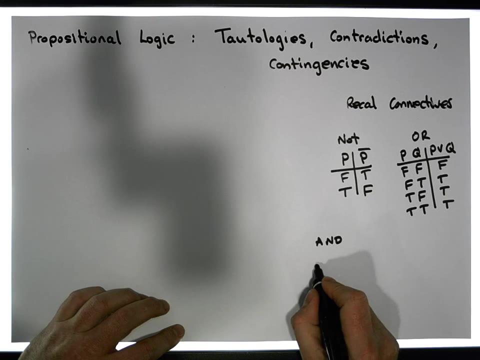 true true false true true. And or is only ever p or q, nor is only ever false when both of them are simultaneously false. So it's false here. everywhere else it's true. We have the and An, and maybe I should write it like this Once again: takes in a p and a q. They're false. 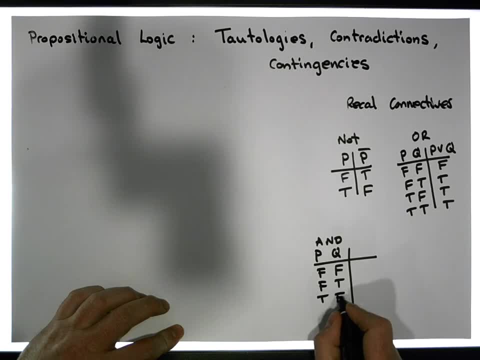 false, false, true, true, false, true, true P and the q: It's only ever true when both of them are simultaneously true. So we have true here. Everywhere else we have false. And then, finally, we have the next important connectives. 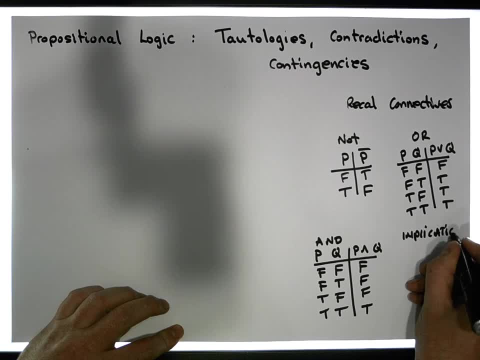 which is implication, Implication. okay, It takes in two propositions Once again. let's just define this as p-q: False, false, false, true, true, false, true true. And p implies q. It looks something like this: It's only ever false when the premise is true. 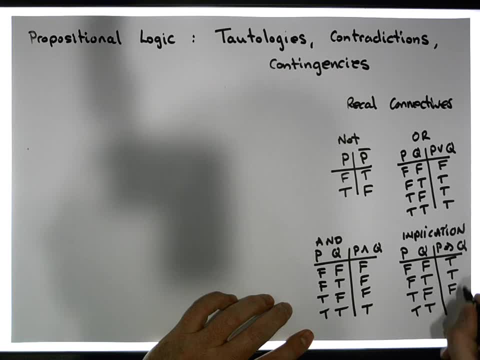 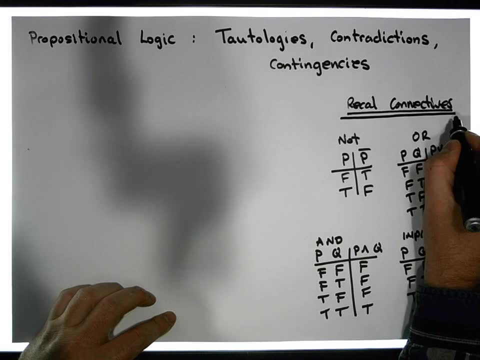 and the conclusion is false. It's only ever false here. Everywhere else it's true, okay. So let's just keep these in mind. These are our connectives, okay, And let me just give you some examples. Let's build some true tables for some propositions. okay, Let's do a simple one, Yeah. 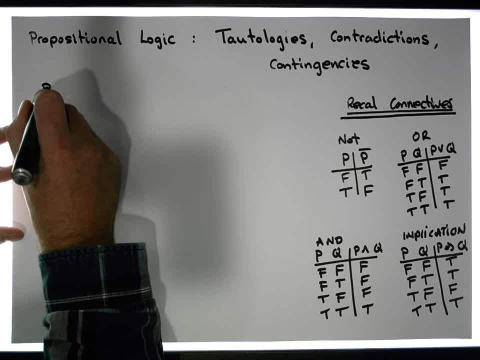 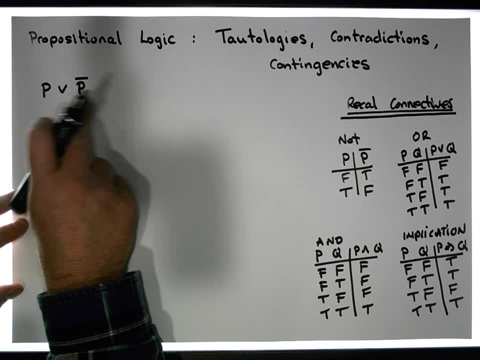 let's say we have the propositional expression p or'd with, not p. okay, So I want to build a true table for this. Let's just keep in mind that the propositions- there's only one proposition in this, It's the proposition p. 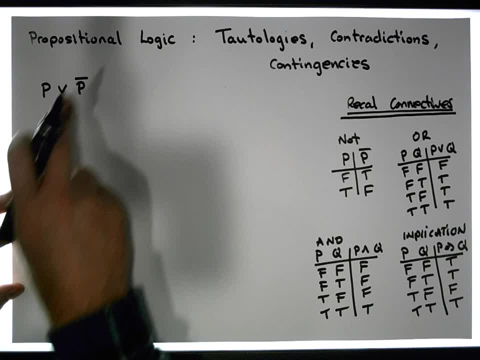 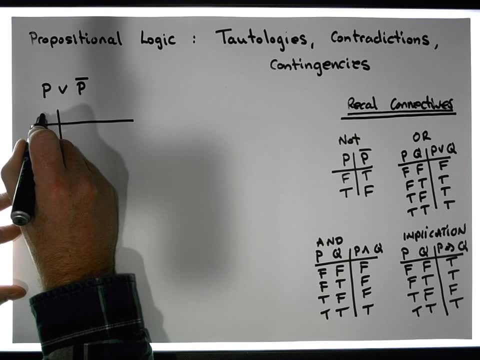 Albeit, there's two connectives, There's an or and, there's a negation, or there's a not. okay, There's still only one proposition here, okay? So I'm going to build a true table for this. I'm going to specify the propositions that are in it down the first column, which is just a. 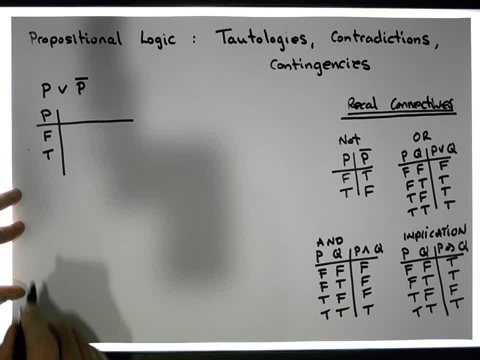 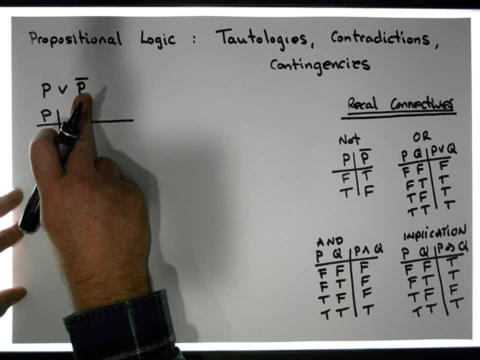 p. The values they could take on is false and true. okay, To build the, or I need the p values, which are already here, but I also need the negation of the p, so I need the, not values. okay, So I need to construct a p-bar column. okay, And by definition, falses go to trues. 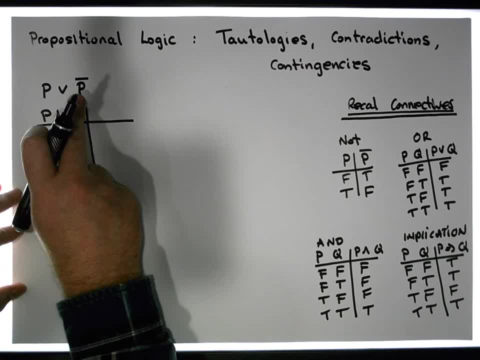 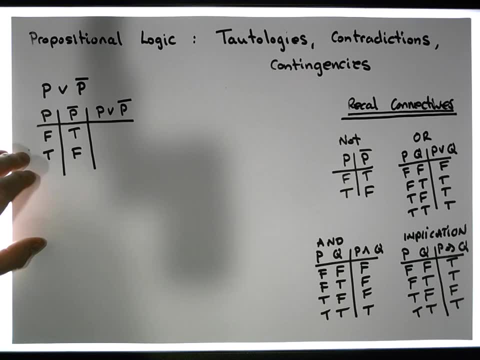 and trues go to false, falses for the negation. Now I have both inputs to the OR. I can construct the OR. so what we have here is P OR, not P as an example, and we know the way an OR works. an OR is only ever false. 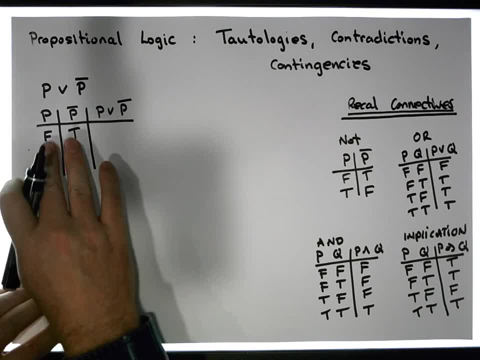 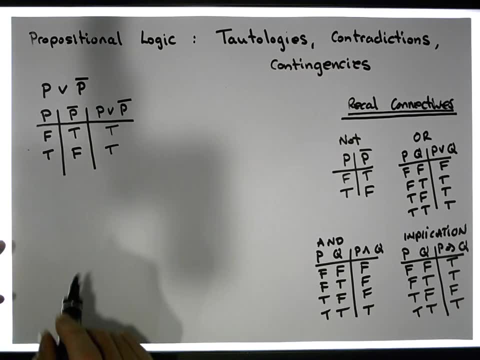 when both of the inputs are simultaneously false, and we can see that the inputs are never simultaneously false here. so what we get is we get a true and a true value. So the important thing here is this: for our definition is that the output of this particular expression under 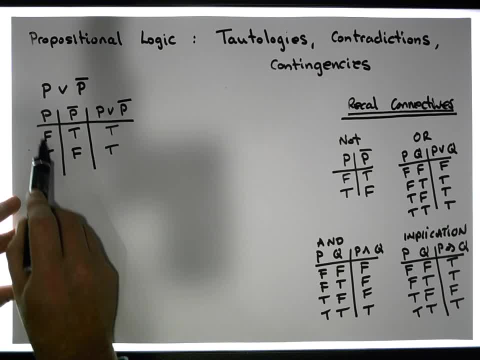 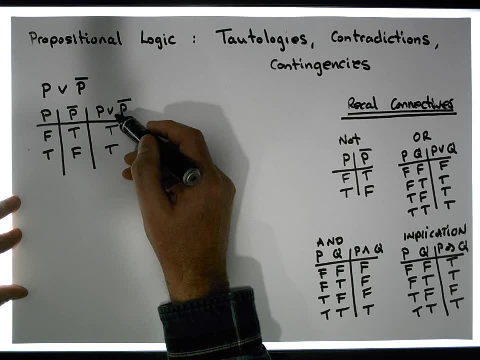 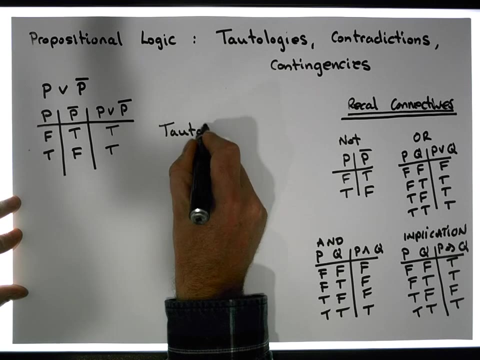 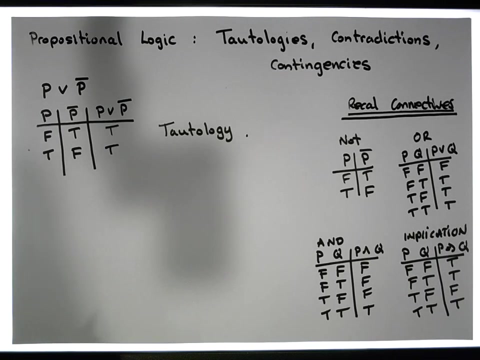 all possible inputs. irrespective of what the input is, the output is always true. and we call a statement a propositional statement that evaluates when its output is evaluated under all possible conditions and that all possible evaluations are true. we call that a tautology. a tautology, okay, tautology, okay. now let's see what's what would be a contradiction, okay, so 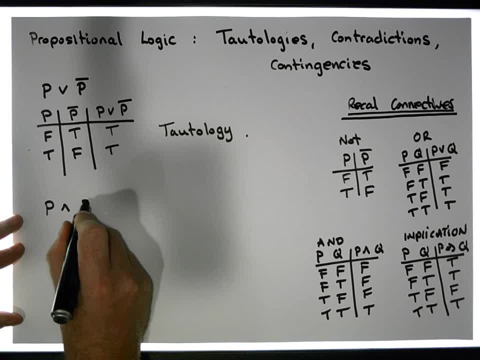 P. another example is P and not P. okay, so let's build a true and a false. So let's build a true and a false. So let's build a true and a false. So that's why we'veって build a clue table for this. Let's see what happens. so the inputs. 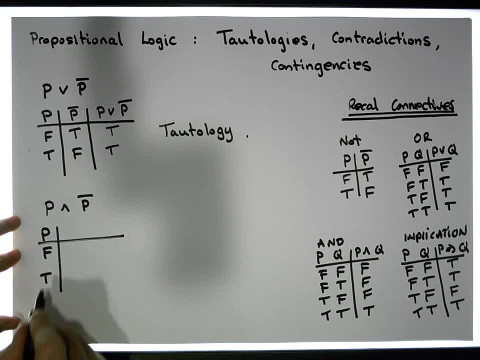 is only one proposition. it's a P, it could be false or keep it true. to do the, and we need to have the values for P, which are already listed here, okay, and we need to have the values for not P, which we don't have listed. so we need to evaluate not P, p well, a false is equal to truths and 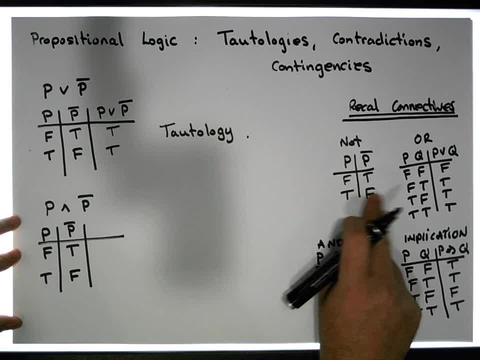 truth goes to false. that's the way the not works, okay. and now we can do the and P, and with not P, not P. okay, and we see an and only ever gives us true, and both of them are similar, Simultaneously true. that's the definition of our and. 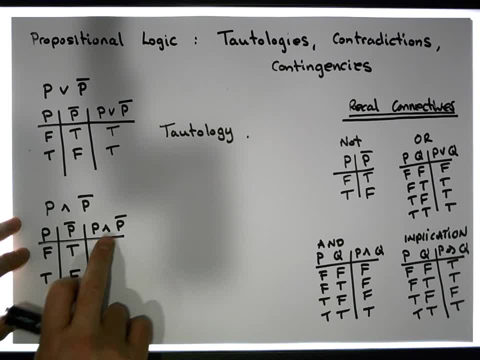 And they're never simultaneously true. the two inputs yeah To the, and they're never simultaneously true. So what we get is we get a false and a false here. So in this example, a very small propositional expression: okay, here. 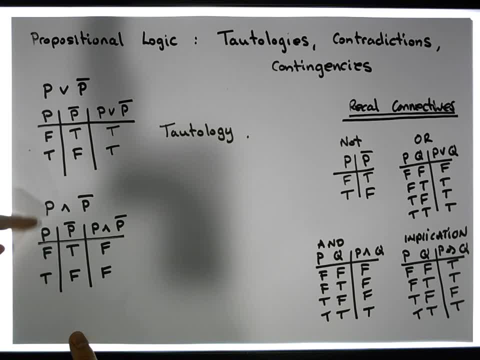 In this example, no matter what the inputs are to the proposition, to the propositional expression, no matter what the inputs are, the output is always false. So in this case here we call this type of proposition a contradiction. Okay, and if you think about it in the real world,